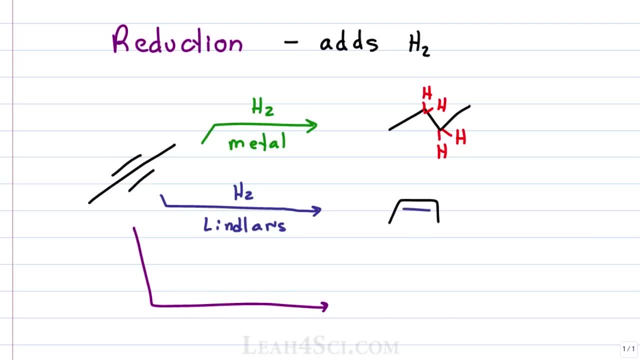 you get a cis alkene. A Lindler's catalyst is a poison catalyst that reacts just like the standard metal, where the metal is reactivated with H2 and a Lindler's catalyst. If you react with H2 and a Lindler's catalyst, the metal grabs the pi bond from the same face and adds the hydrogen to the 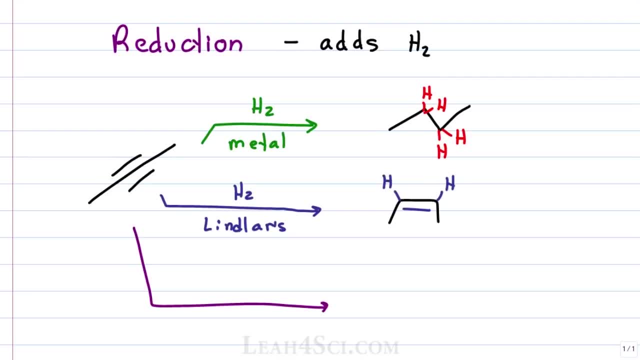 same face of the molecule. This would be considered a syn addition for alkenes or a cis alkene product. when starting with an alkyne, When subjected to dissolving metal reduction using something like sodium in liquid ammonia, keep in mind that a neutral sodium is a radical. It only has 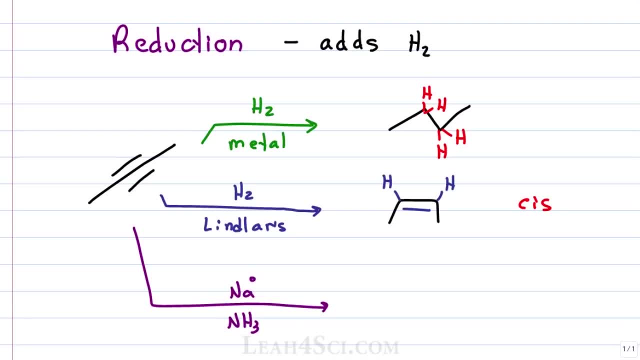 one electron in its valence. This will give it a radical intermediate. The electrons want to go as far from each other as possible. and what does the final product look like? when electrons are as far from each other as possible, We get a trans alkene. Do not confuse the NaNH3 with NaNH2.. Sodium here. 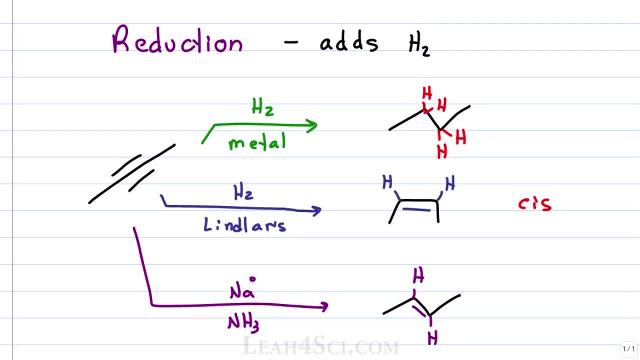 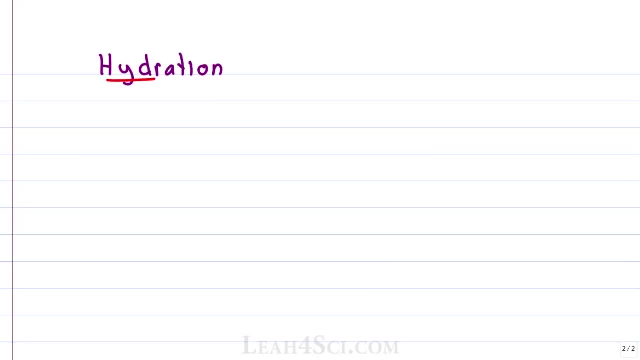 is a neutral radical metal where the NaNH2 is Na plus and amide NH2 minus, which acts as a very strong base. Here the NH3 is simply a solvent to give us the trans product. Hydration reaction is where we hydrate the alkyne and add an H2O. Alkenes could be hydrated with an acid catalyst. 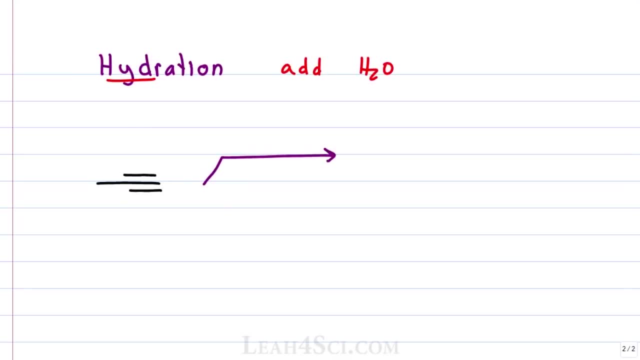 or oxymercuration. to give you a Markovnikov product For alkynes, we combine the two using HgSO4 and H2SO4 in water for an acid catalyzed hydration. Just like the alkene reaction, we break a pi bond and put the OH on the more substituted carbon atom. But since the alkyne 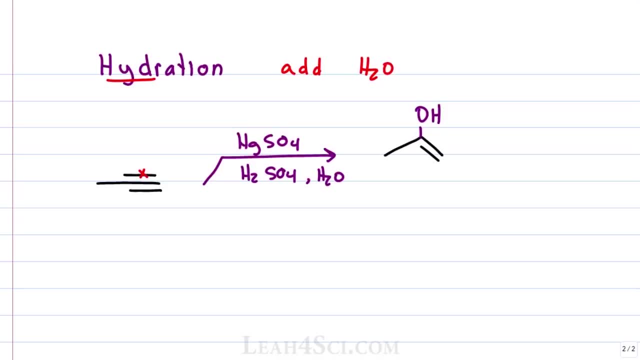 started with two pi bonds. we still have one more For a product that has both an alkene and an alcohol, giving me an enol. This is not a very stable intermediate and will undergo ketoenol tautomerization to isomerize into the keto form. 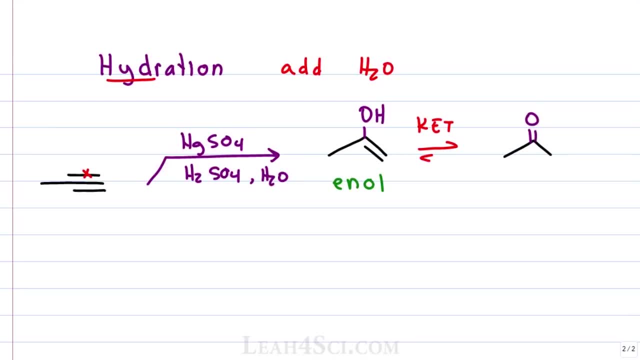 in this case, a ketone Hydroboration of all kinds works very similarly, but instead of BH3, you might see different boron containing reagents such as R2BH, SIA for disiamyl 2-borane, or even 9-BBN. We still have the same conditions dissolving it in THF for step 1 and step 2 is. 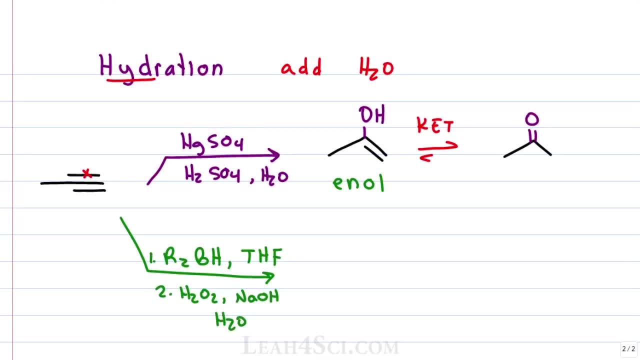 followed up with peroxide, base and water. As with oxymercuration, we first get an enol product, but this time the alcohol adds to the less substituted carbon, and this too will undergo ketoenol tautomerization, in this case giving us not the keto form, but the aldehyde form. 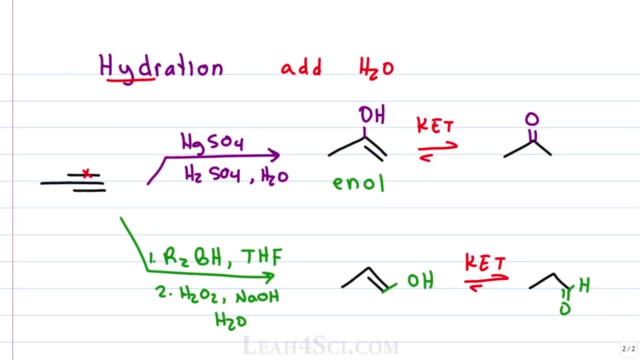 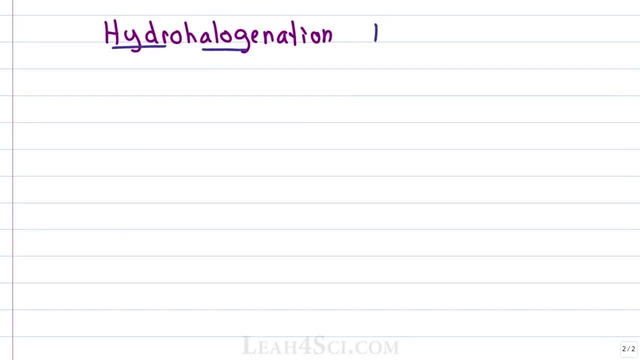 For more on ketoenol tautomerization, stability and mechanism, see the video linked below. Hydrohalogenation, as the name implies, adds a hydrogen and a halogen HX, where X could be fluorine, chlorine, bromine or iodine. We'll use terminal alkynes so that we can pay more. 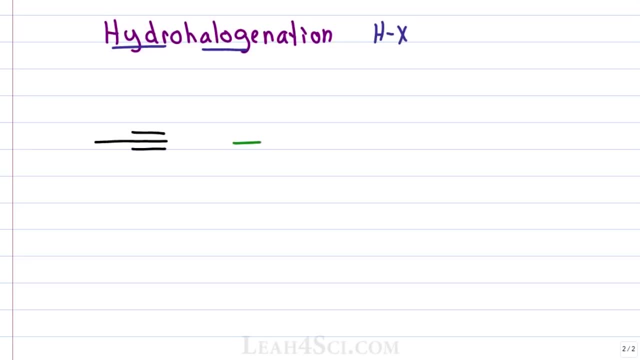 attention to Markovnikov and anti-Markovnikov products. If you react a terminal alkyne with HX, for example HBr, you break the pi bond. add the hydrogen to the less substituted position and the halogen to the Markovnikov or more substituted position. 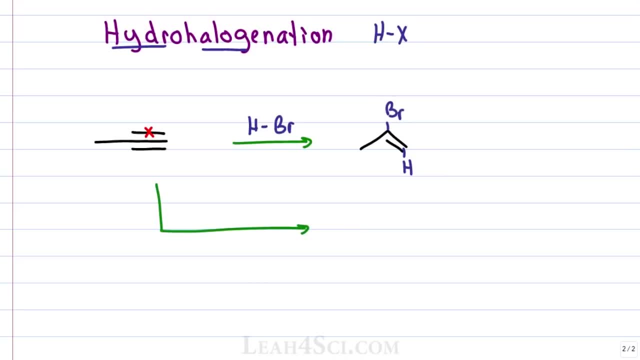 This is a simple process to get rid of the hydrogen and the hydrogen to the less substituted position. This is a simple process to get rid of the hydrogen and the hydrogen to the less substituted position. This reaction will typically take place in excess hydrohalogen, for example, excess HCl. 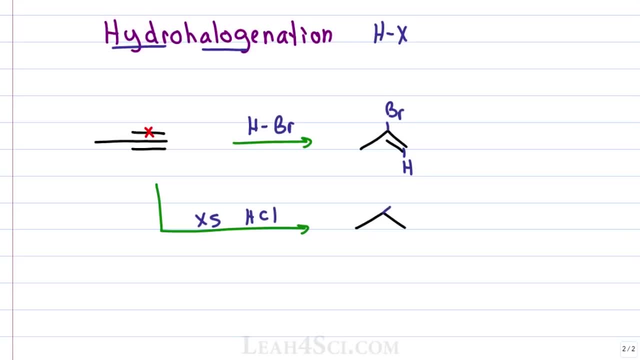 so that both pi bonds break and both halogens add to the more substituted carbon. Once again the product follows Markovnikov's rule. but for excess reagent we get a geminal dihalide. I think of it as a gem. if I have a few, I wanna keep them close. I wanna keep them on the same. 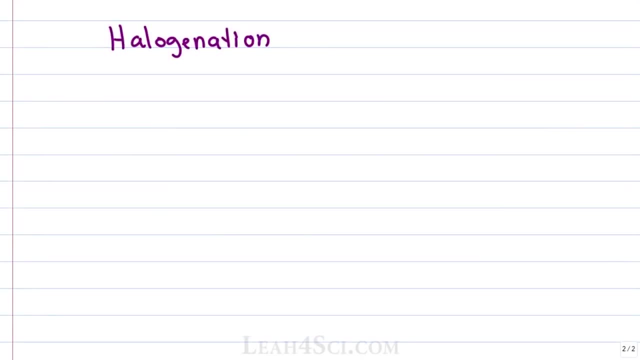 carbon Halogenation is very similar, except that we're using X2 instead of HX to add two halogens per reaction. If you react an alkyne with X2, such as Br2, you simply break the pi bond and put one halogen on each carbon. As with hydrohalogenation, this is typically carried. 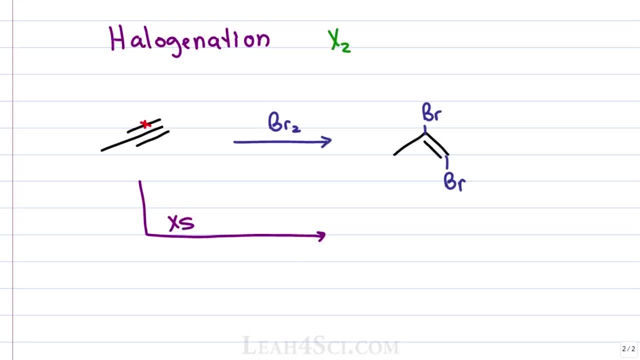 out with excess reagent where you're providing more than enough halogen to add to your pi bonds. For example, if I react it with excess HCl2, I break both pi bonds and put two halogens each on the carbons that used to be triple bound, For a total of four halogens per reaction. 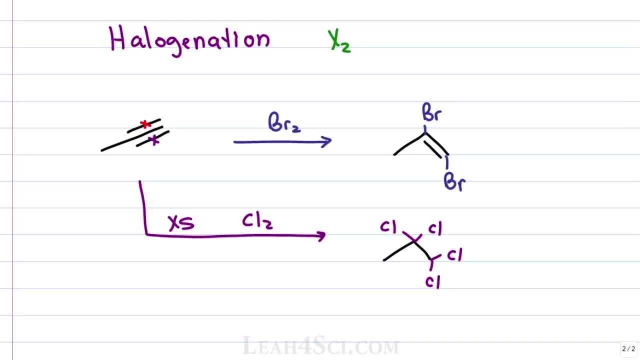 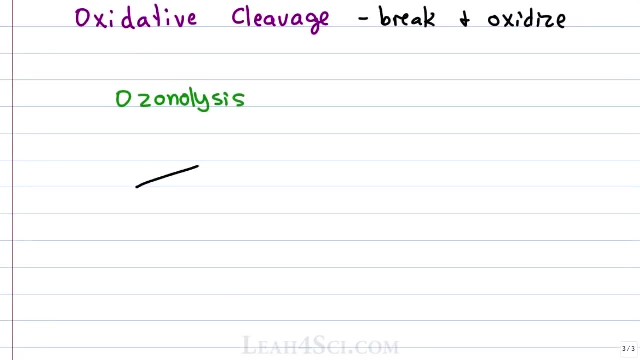 four halogens added, two per pi bond being broken. Oxidative cleavage is when you break the bond and add oxygen to that same carbon. You likely covered ozonolysis and potassium permanganate KMnO4 oxidation. Ozonolysis uses O3 or ozone to cleave not only the pi bond but also the sigma bond and 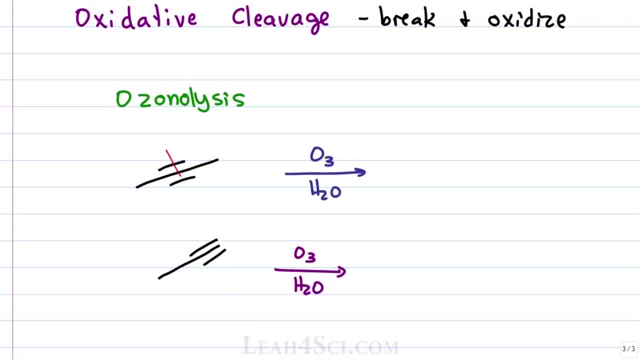 this is followed by H2O. The trick here is to cut the molecule right between the pi bonds and add oxygen to the molecule. You can also use a double bound O and a single bound OH for this reaction. In this case, the carbon will be separated out for every break The products. 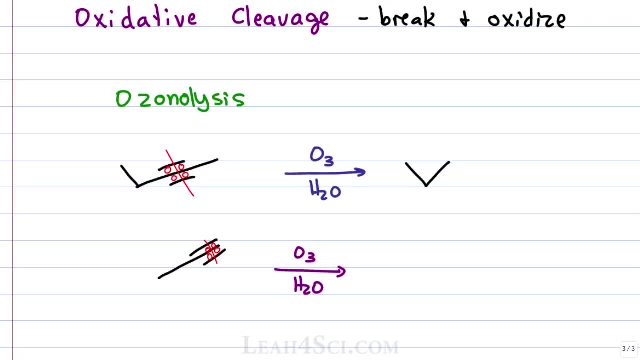 will be different if you're starting with an internal or terminal alkyne. For an internal alkyne, you'll get two carboxylic acids. Start out by redrawing the carbon skeleton exactly as you see it, but leaving a gap where you cleave the molecule. Then simply add in a double bound, O and. 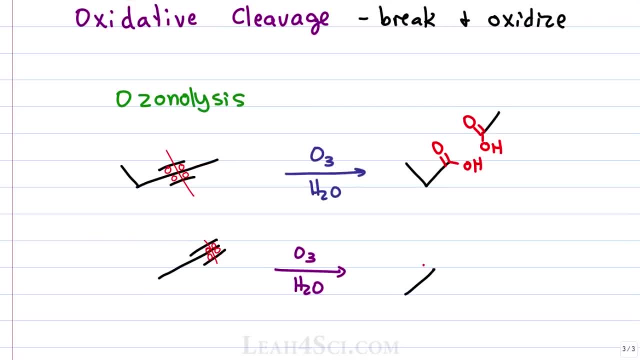 a single bound OH for the carboxylic acid. So we have two carbons. so we put a carboxylic acid on the end For the single carbon it'll start out forming a carboxylic acid, in this case formic acid, but this will quickly decompose to give you. 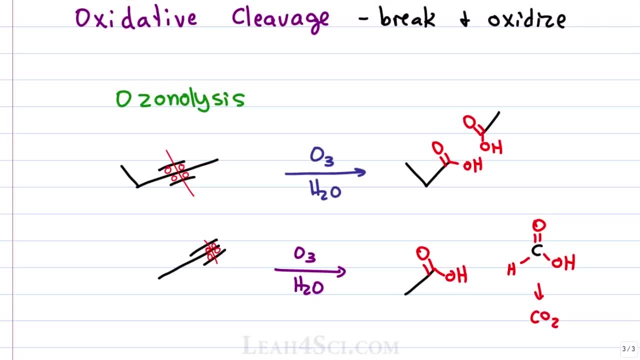 carbon dioxide, which is a fully oxidized carbon. Some professors will teach formic acid as the product, others will teach CO2, so make sure you figure out which one you're required to know before you memorize it. Permanganate oxidation can be carried out under different conditions. 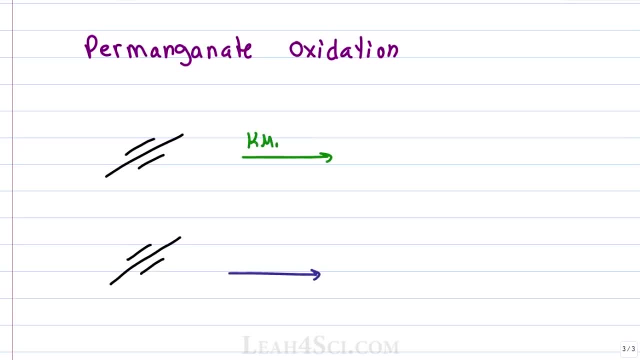 So what we're gonna do is we're gonna break down the pi bonds into two completely different products. Reacting an alkyne with potassium permanganate under weaker or neutral conditions will only break the pi bonds, but not the sigma bonds. This will give us a product that initially 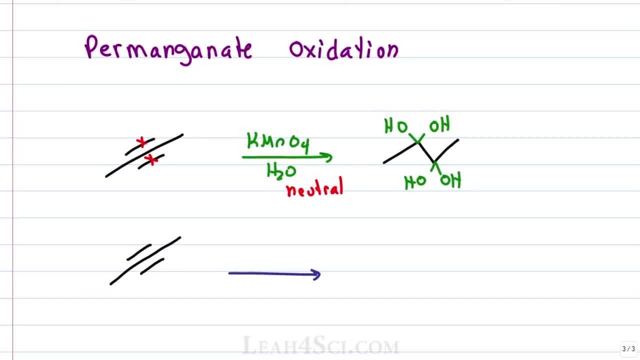 has one alcohol added to each carbon for each pi bound broken. This gives us a total of four alcohols, which is very unstable, and so the molecule will rearrange, kicking out water and turning each carbon into one. The final product is a diketone. When carried out under hot basic conditions. 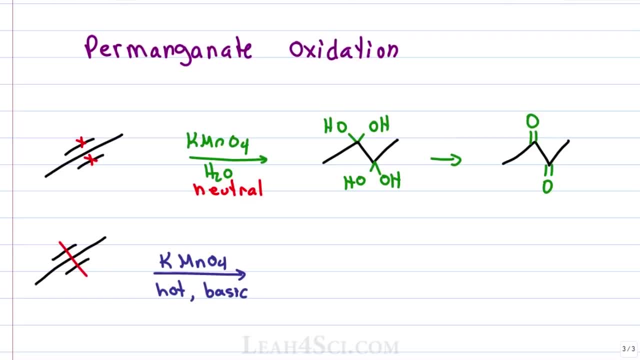 you get a more extreme reaction and we get a similar cleavage to ozonolysis, where you break it right down the middle and add an oxygen to each side of the cleavage for every pi bond that was broken. The only difference is that under basic conditions you can't form a carboxylic acid, but 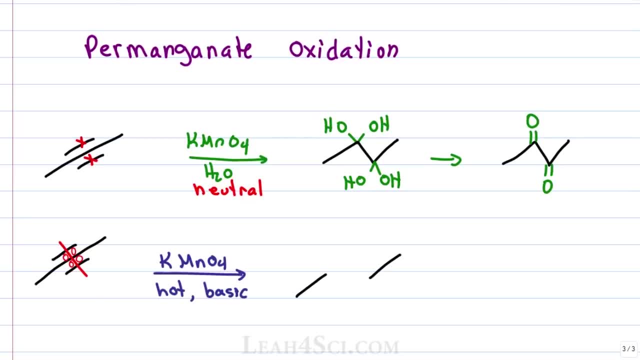 instead you have the deprotonated conjugate base. Redraw the skeleton exactly as you see it, so that you have a carboxylic acid in the middle and a carboxylic acid in the middle and a carboxylic. 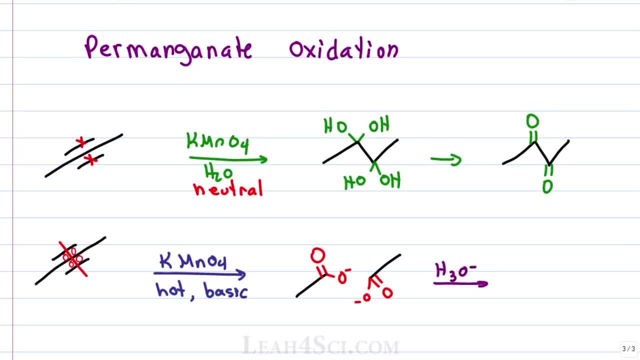 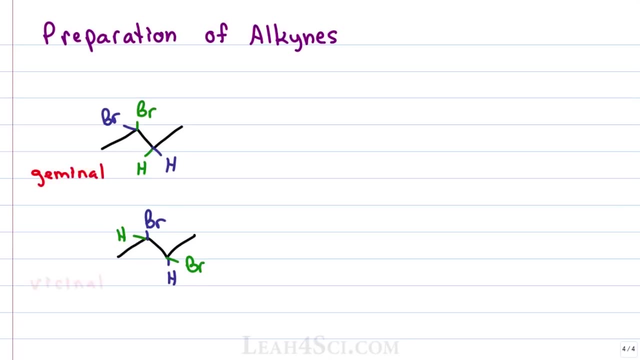 acid in the middle. If you react this with a mild acid, in this case, we'll show H3O plus. each molecule will be protonated for a carboxylic acid final product. In addition to reacting alkynes, you also have to know how to make them. An alkyne can be formed from a geminal or vicinal. 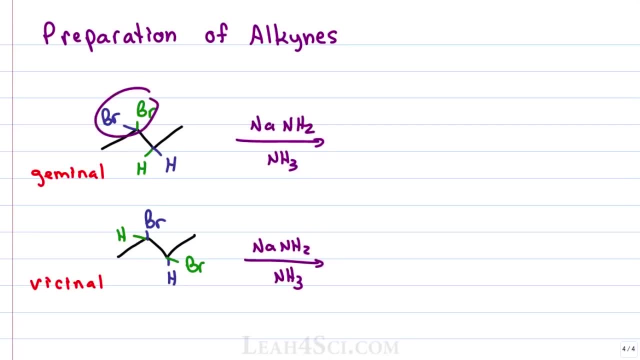 dihalide, where geminal has two halogens on the same carbon and vicinal has them in the vicinity on neighboring carbons. The alkyne is formed by two elimination reactions using excess strong base sodium amide, NaNH2, dissolved in liquid ammonia. Vicinal and geminal dihalides will give you the same exact product. 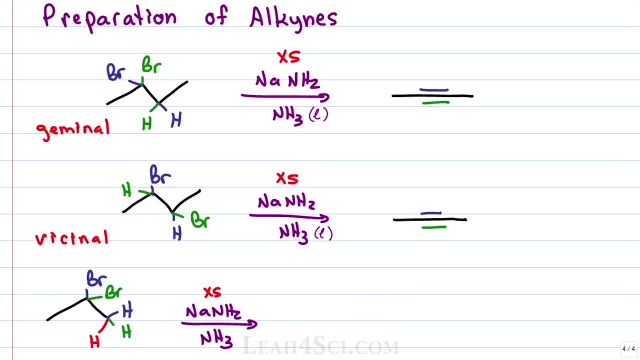 Terminal alkynes present a tricky extra step. Each NH2 minus will grab a hydrogen and eliminate a halogen, giving us an expected alkyne. but the problem is we still have a terminal acidic hydrogen atom and another NH2 minus in solution will reach for that hydrogen and 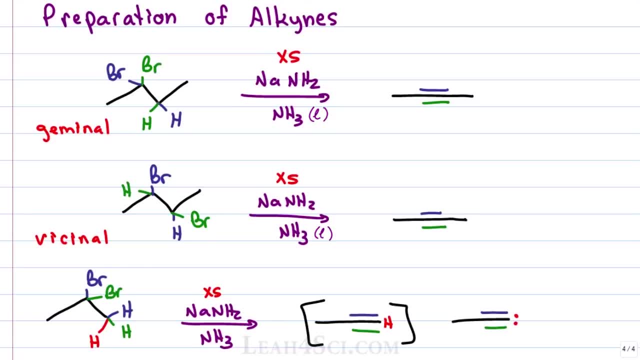 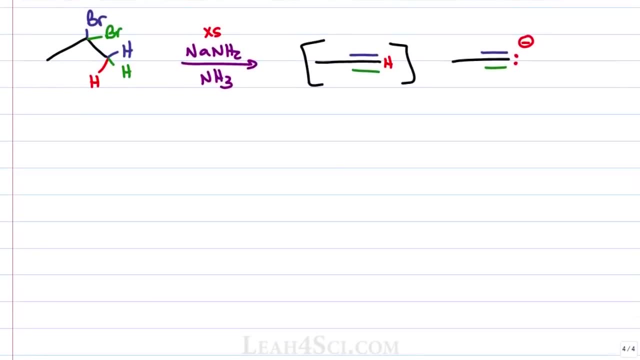 deprotonate the alkyne. This gives us the alkanide anion For a two carbon molecule, that's the acetylide anion. If your goal is alkylation, you're okay, but if your goal is simply to form the alkyne, you have to react this with water so that the very strong base 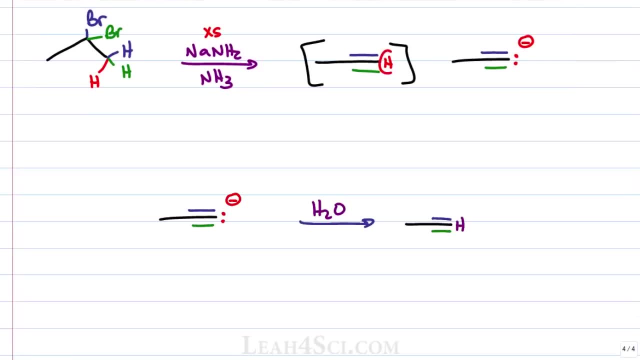 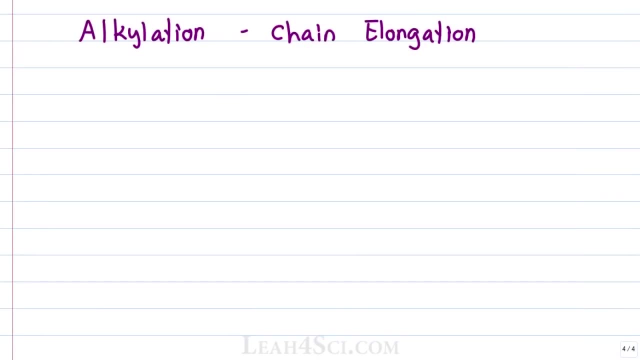 can deprotonate the water molecule and regain that hydrogen atom. This is a very useful reaction in synthesis and retrosynthesis because it gives you a way to do chain elongation to create a longer carbon chain. when you're starting with something small, Terminal alkynes have an acidic terminal hydrogen and when reacted with a strong base like sodium, 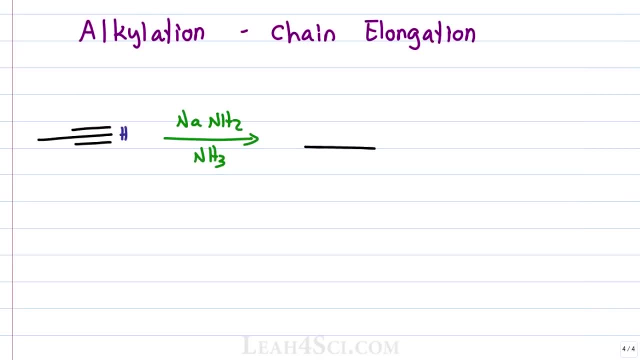 amide in ammonia, the amide will deprotonate the alkyne and give us the alkanide anion. This anion makes a very good nucleophile for an SN2 reaction because the lone pairs can simply attack a carbon, kick out the leaving group, giving you a longer chain which you can then 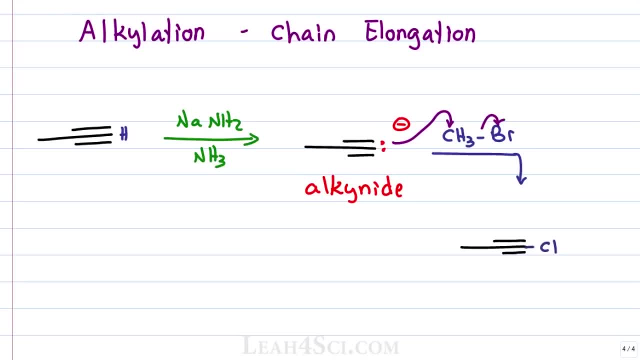 take and subject to any of the reactions we looked at before and introduce all sorts of functional groups and reactivity. This concludes the alkyne shortcut video. I hope this video helps you quickly recognize and understand the patterns for alkyne reactions. Make sure you study these.